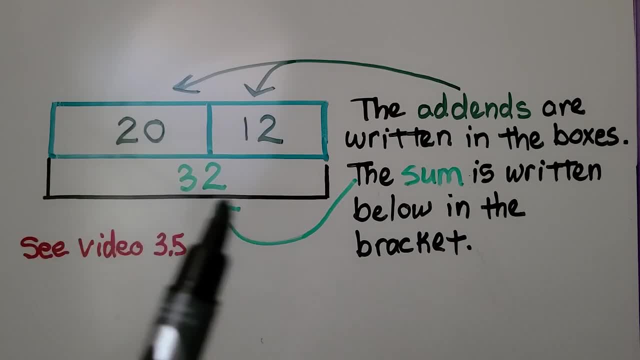 boxes and the sum is written below in bracket. You can even find it written down here below the bracket. And we learned about these back in video 3.5 when we learned about related addition and subtraction facts. That video is in the description, in case you need a link, And bar models or bar. 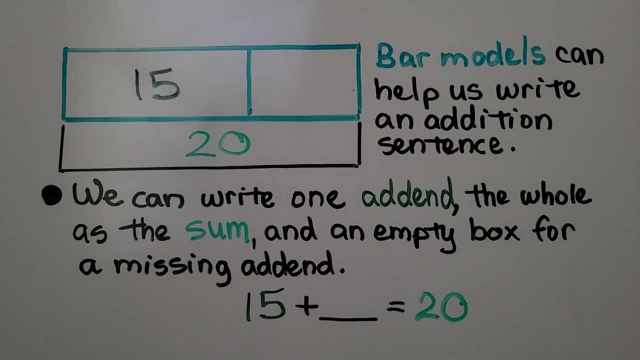 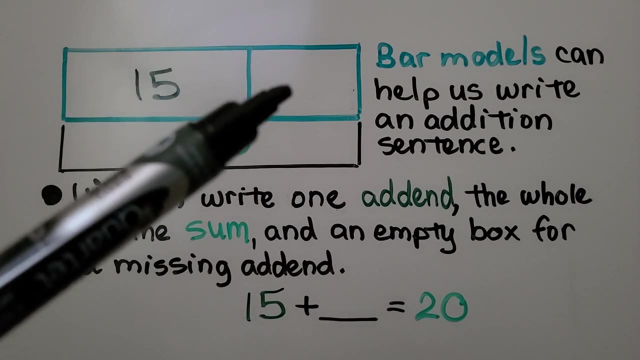 graphs can help us write an addition sentence. We can write one add-in, the whole as the sum, and an empty box for the missing add-in. If we have 15 plus something, we write a 15 here, We leave this box empty, and if it's equal to 20, we write the 20 by the bracket. That would be 15. 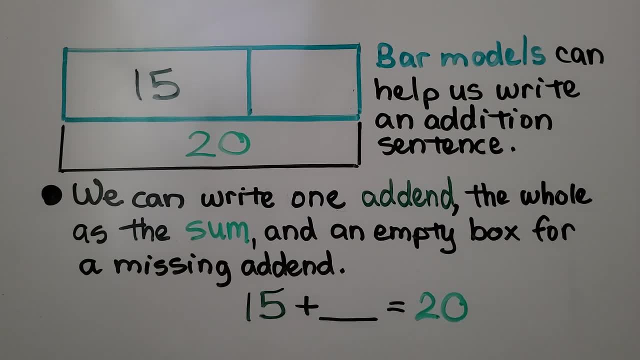 plus, some number is equal to 20.. Do you know what that would be? We can count on from 15.. 15,, 16,, 17,, 18,, 19,, 20.. 15,, 16,, 17,, 18,, 19,, 20.. 15,, 16,, 17,, 18,, 19,, 20.. 15,, 16,, 17,, 19,, 20.. 15,, 16,, 17,, 19,. 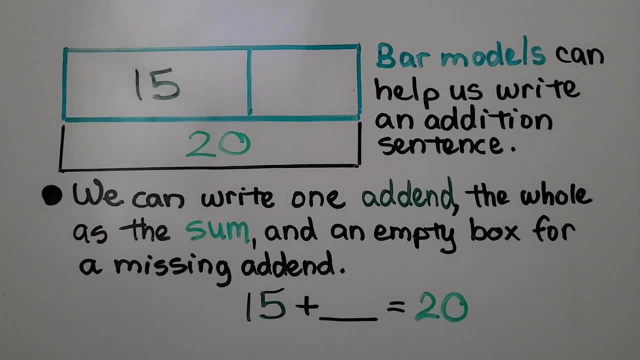 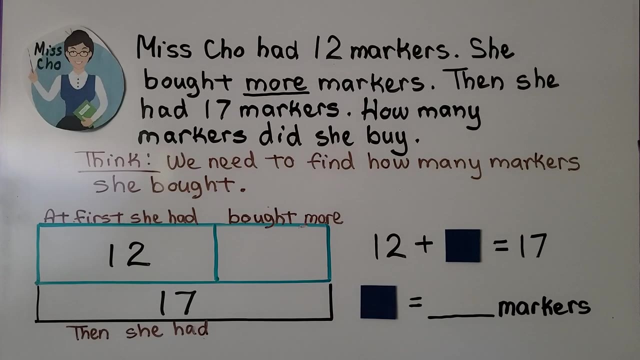 17,, 18,, 19,, 20.. That would be 5.. 15 plus 5 is equal to 20.. The bar model helped us to write the addition sentence so we could solve it. Miss Cho had 12 markers. She bought more markers Then she. 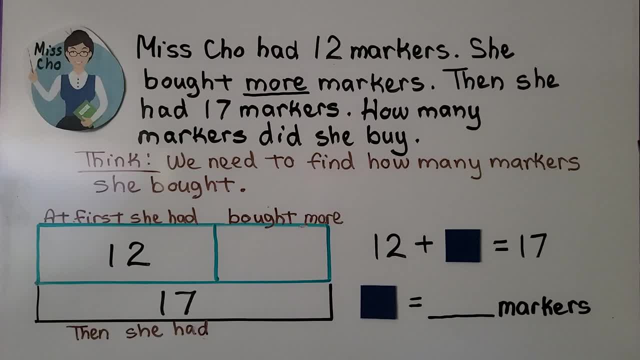 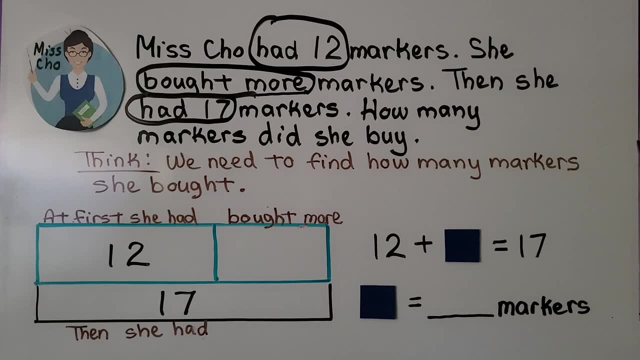 had 17 markers. So how many markers did she buy? And we think we need to find how many markers she bought. We can circle the important ones. We can circle the important ones. We can circle the important information. She had 12 at first. She bought more, We don't know how many more Then. 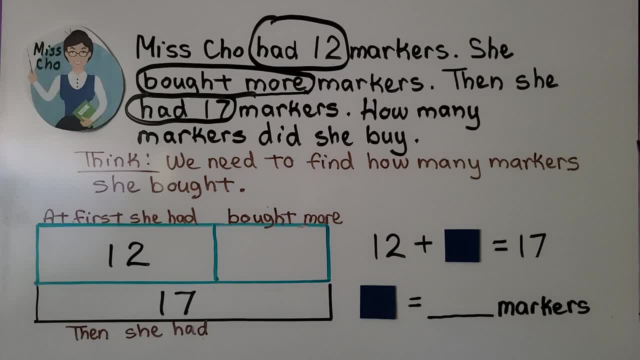 she had 17.. We can write an addition sentence: 12 plus some number is equal to 17. And we can use a little square or any shape really, to take the place of the unknown number. We can start at 12 and count on to 17.. 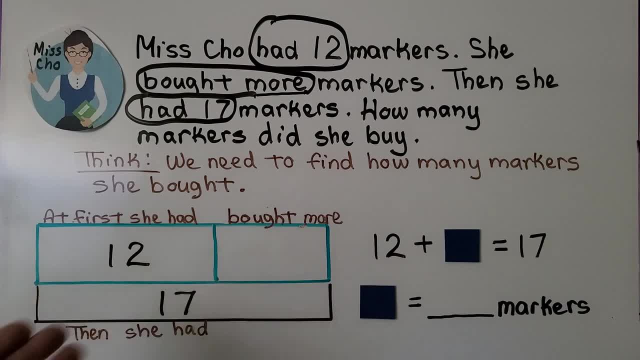 12,, 13,, 14,, 15,, 16,, 17.. That's 5.. That means she bought 5 more. 12 plus 5 is equal to 17.. That means this little square is equal to 5 for 5 markers. 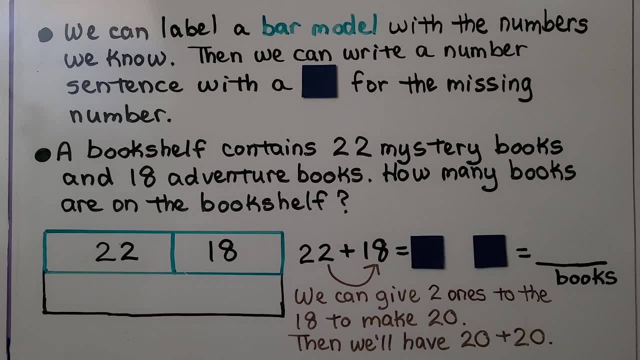 We can label a bar model with the numbers we know. Then we can write a number sentence with a square for the missing number. Here's our problem. A bookshelf contains 22 mystery books and 18 Adventure books. How many books are on the bookshelf? So there's 22 mystery, 18 Adventure. We need to know how many. 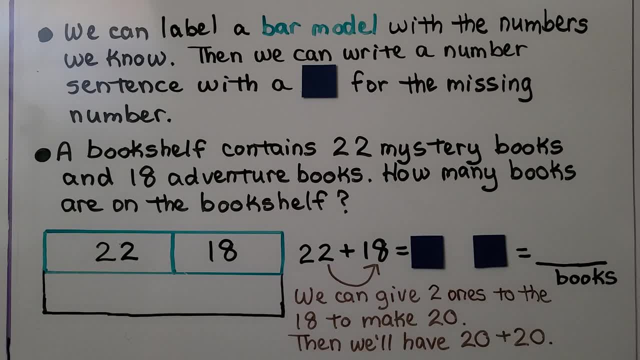 there are as a total. We can write the addition sentence: 22 plus 18 is equal to this square. We think 18 only needs two ones to be 20, so we can give two ones from here to the 18 to make a 20,. 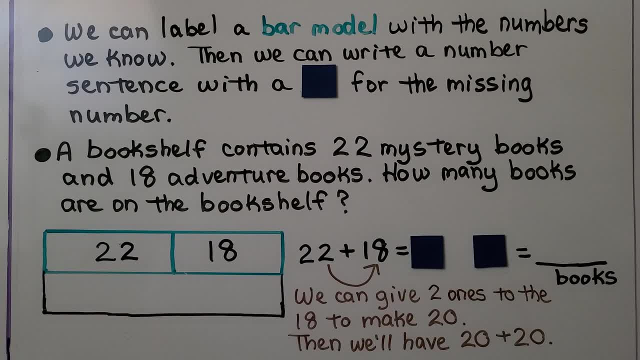 and now that's 20 plus 20.. That's easy to add. Do you know what 20 plus 20 is equal to? If you said 40,, you're right. That means this square is equal to 40 books. There were 40 books. 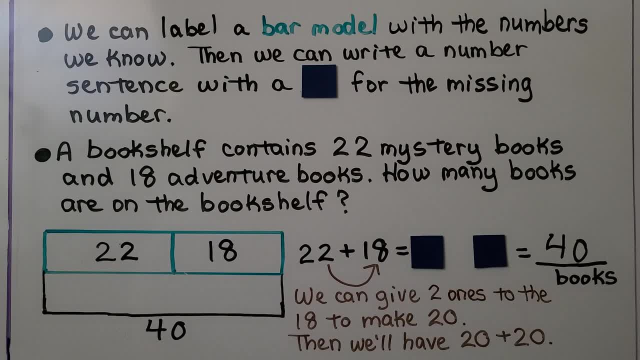 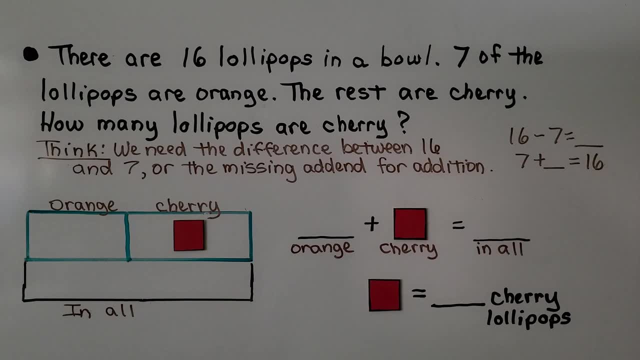 on the bookshelf. There are 16 lollipops in a bowl. Seven of the lollipops are orange and the rest are cherry. So how many lollipops are cherry? We think We need to find the difference between. 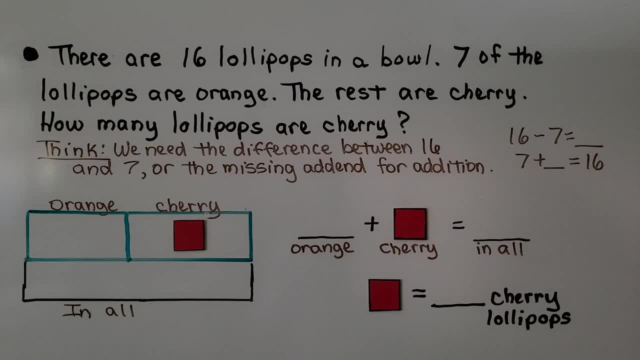 16 and 7.. There's 16 in all. 7 of them are orange. The difference would be the cherry. We can also think of it as a missing add-in for addition, because addition and subtraction are less than or equal to. So let's add a negative tangent for addition and subtraction. 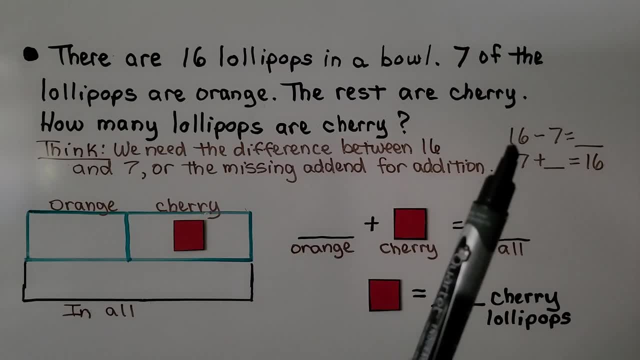 subtraction are related. We can think of it as 16 minus 7 is equal to the number of cherry. or we could think 7 orange plus the number of cherry is equal to 16.. In our bar model we know there were 16 in all. We also know that 7 of the lollipops 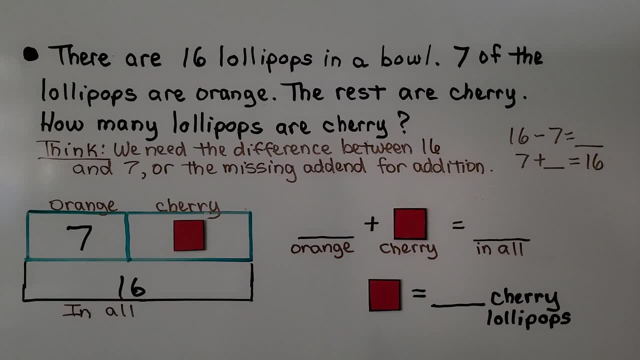 are orange. Using a related addition sentence to subtraction, we have 7 plus some number that is cherry is equal to 16. in all, 7 plus the cherry is equal to 16.. We need to figure out what this number is, that if we add it to 7, it will equal 16.. Do you know? 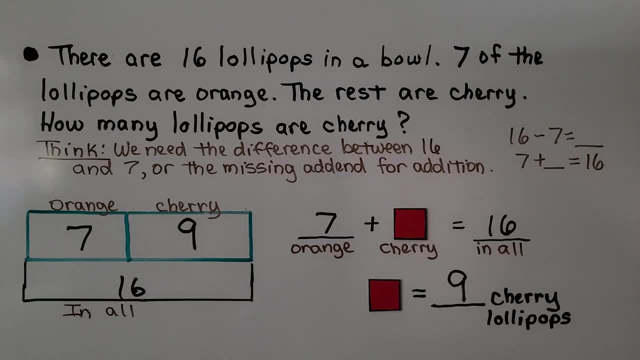 Okay, If you said 9, you're right. 7 needs 3 more to be a 10.. Now we're at 10, we need 6 more to be 16.. We add the 3 and the 6 together, that's 9.. That's 9. cherry lollipops in the. 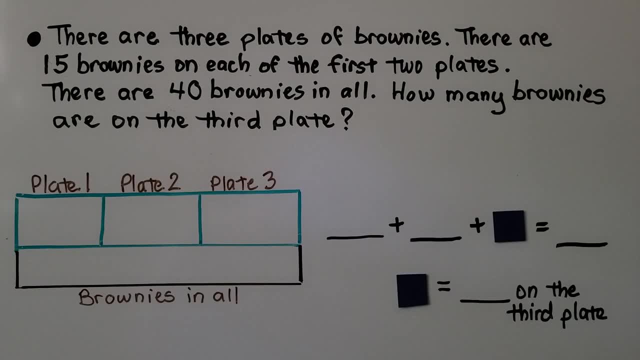 bowl. This problem says: there are 3 plates of brownies. There are 3 plates of brownies. There are 3 plates of brownies. There are 15 brownies on each of the first 2 plates. There are 40 brownies in all. How? 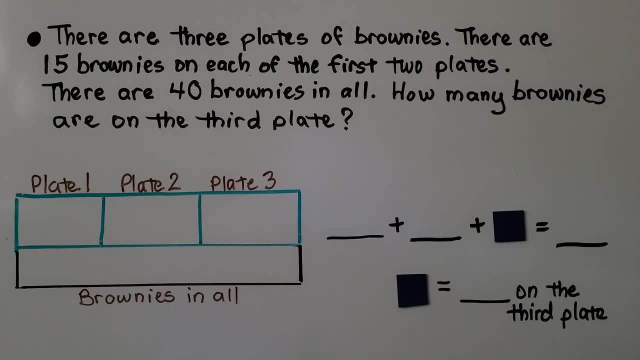 many brownies are on the third plate. So now we have 3 boxes in our bar graph. We have plate 1, plate 2, plate 3, and they're equal to how many brownies in all We know. it says: 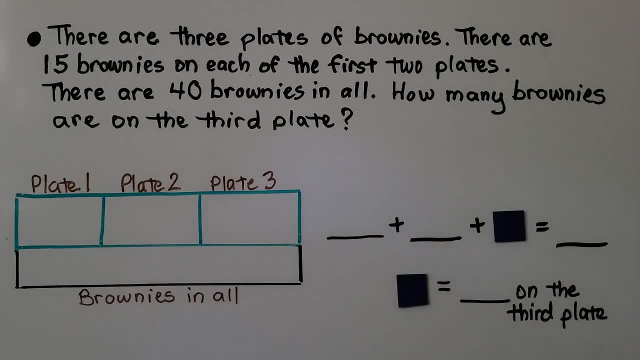 there are 15 brownies on each of the first 2 plates. That means there's 15 on this plate, 15 on this plate and 15 on this plate, And it's telling us that there's 40 brownies in all. We need to find this missing addend. 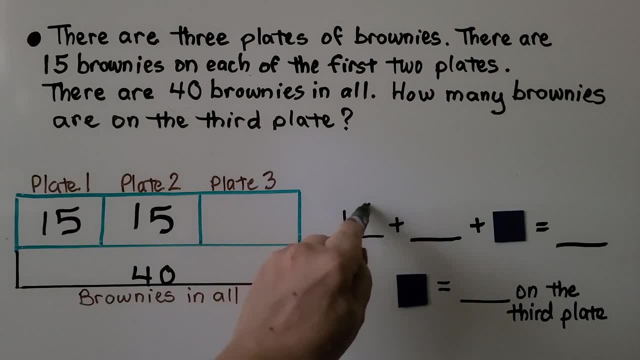 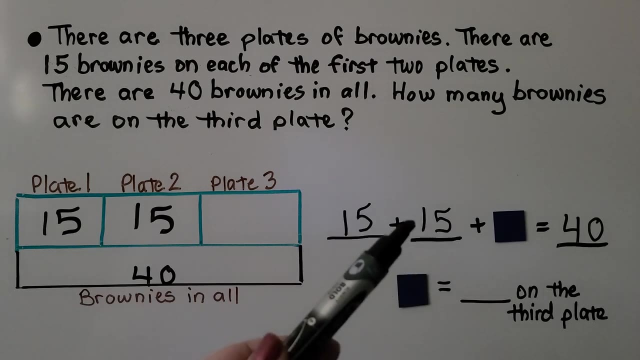 We can write an addition sentence: 15 plus 15 plus that square is equal to 40.. We can add 15 plus 15.. We've got: 5 plus 5 is 10, and another 10,, that's 20, and another 10,. 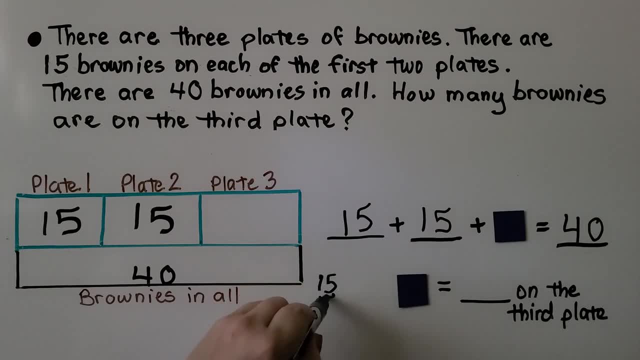 that's 30. We can double check it by stacking them. 5 plus 5 is 10.. We regroup the 10, put the 0 down and we have 3 tens. So that's 30. But there's 40 in all. So how many could? 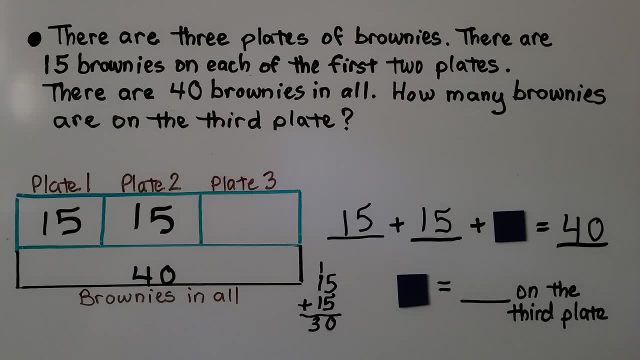 be here. 30 plus some number is equal to 40. If you said 10, you're right. 30 plus 10 is equal to 40. There must be 10.. 10 on the third plate And our little square in our number sentence. our equation is: 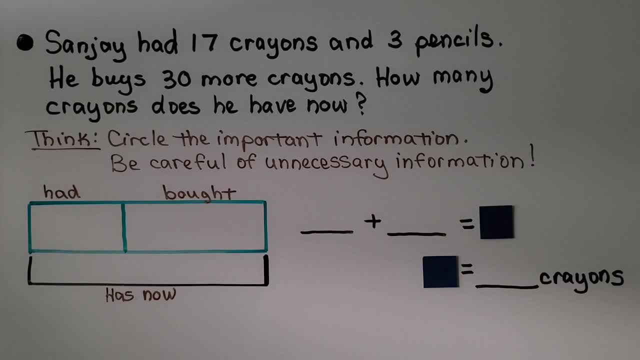 equal to 10.. Sanjay has 17 crayons and 3 pencils. He buys 30 more crayons. How many crayons does he have now? We think Let's circle the important information. What are we looking for? We're looking for how many crayons he has now. He has 70 new crayon set diligently. He's already been given one that's most valuable to him. That's being reported wrongly. I've got 10 more Nous, 20 more. These can't be roomed in. My brother's show is on right detail. That thinks too much. He just went to leftovers for the orderl hospitals. Eat the moment once. 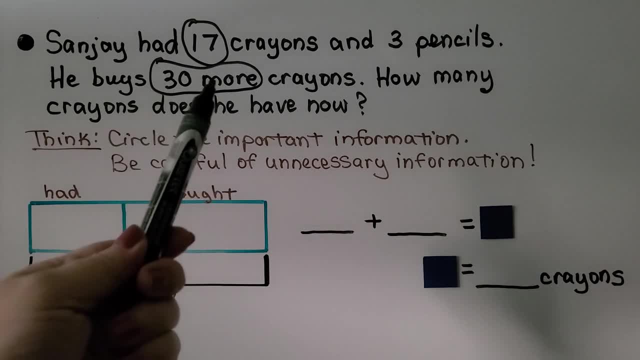 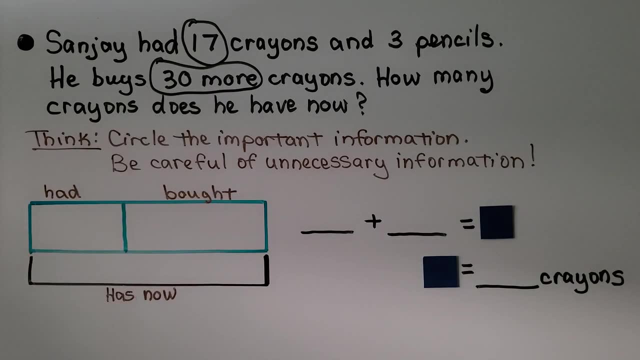 has 17 crayons, he buys 30 more. That means we're going to add 17 and 30. We have to be very careful if there's unnecessary information. that's information that's not needed. Do we need to know he has three pencils? No, we don't. It's not important. We know he had 17 crayons He bought. 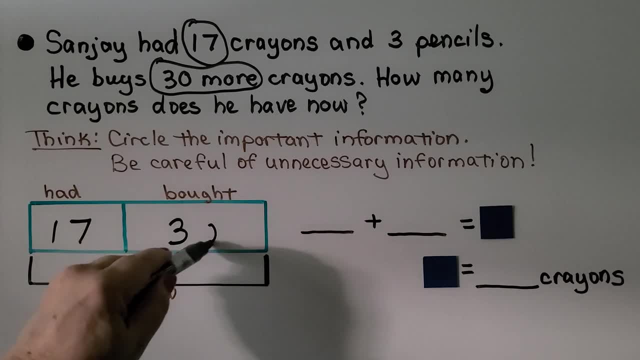 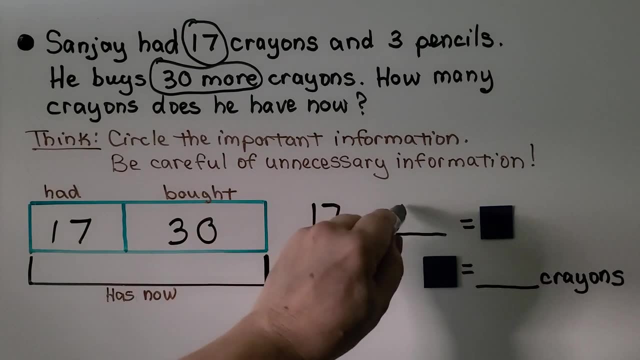 30 more. So how many does he have? now We can write a number sentence, an equation: 17 plus 30 is equal to some number. We have 17 and we're just adding three tens to it. We could do this. 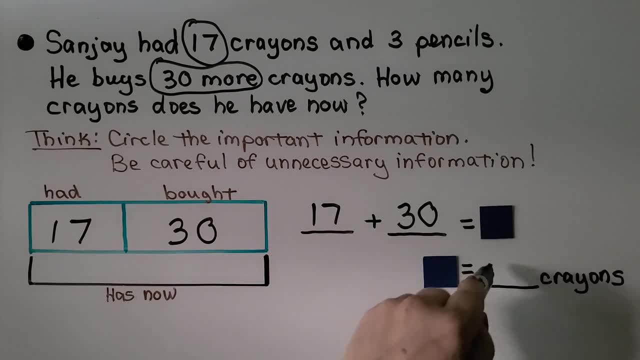 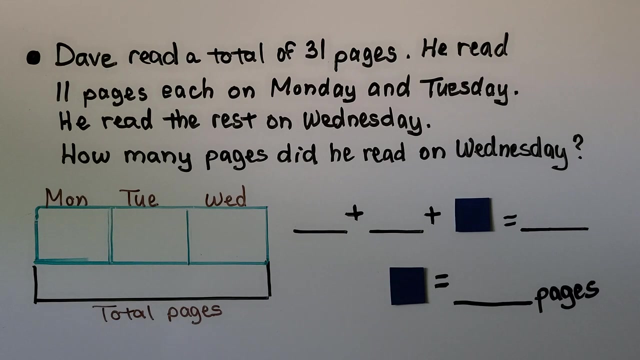 with mental math. One ten and three tens is four tens. We still have the seven ones. That means he's got 47 crayons And the little square is equal to 47.. Dave read a total of 31 pages. He read 11 pages each on Monday and Tuesday. He read the rest on. 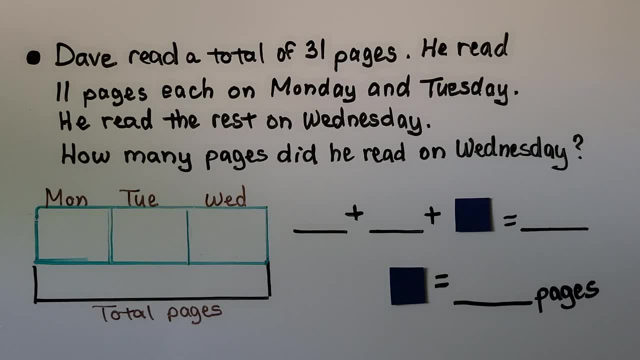 Wednesday. So how many pages did he read on Wednesday? Well, we know he read a total of 31.. We know he read a total of 31 pages on Monday and Tuesday. He read the rest on Wednesday. No, he read 11 pages each on Monday and Tuesday. So our bar model has three boxes here. He read 11.